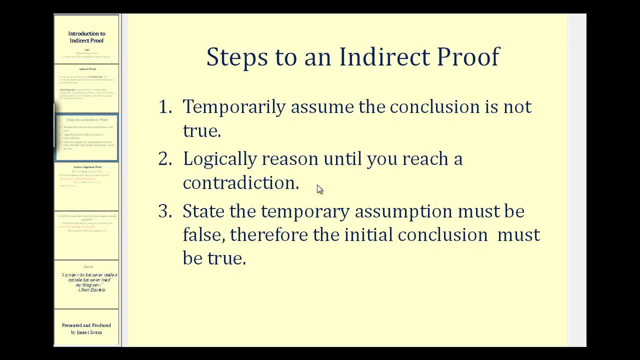 and then we logically reason until we reach a contradiction, and then we finish by saying that the temporary assumption must be false. therefore the initial conclusion must be true. Let's take a look at a couple basic examples of indirect proof so we get a better feel for this type of proof. 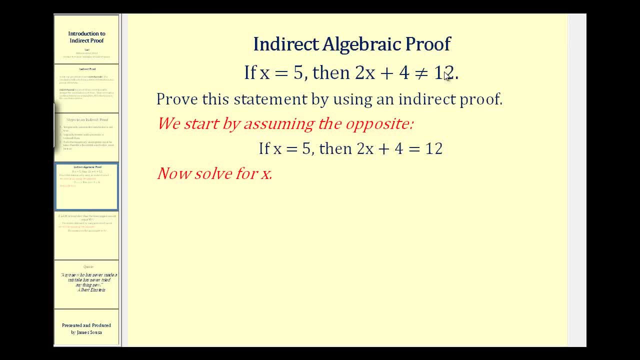 We'll first take a look at an indirect algebraic proof. We want to prove that if x equals five, then two x plus four cannot equal twelve. So by following the steps of indirect proof, we'll start by assuming that the opposite is true meaning: if x 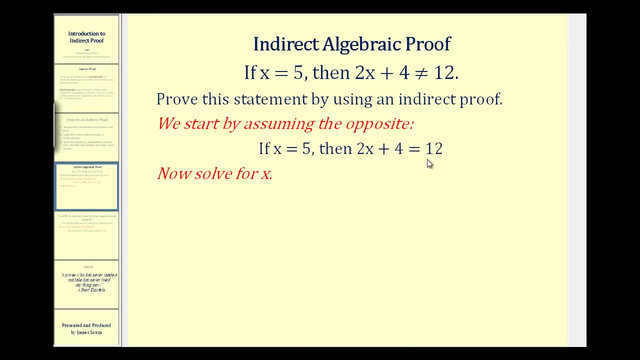 equals five, then two x plus four is equal to twelve. Now what we'll do is go ahead and solve this equation and then hopefully reach a contradiction. Let's give it a try. So we're going to solve: two x plus four equals twelve. 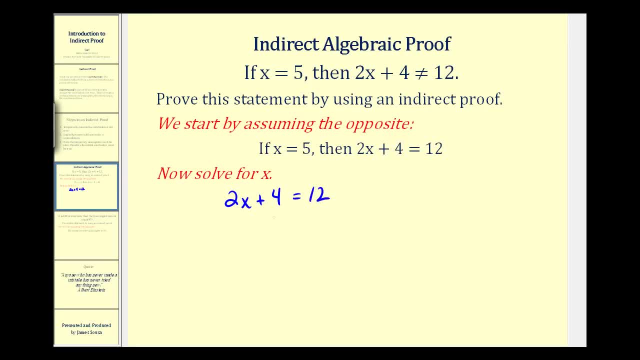 So the first step would be to subtract four on both sides, So we'd have two x equals eight, and this would be from the subtraction property of equality. Next step would be to divide both sides by two. This gives us x equals four. 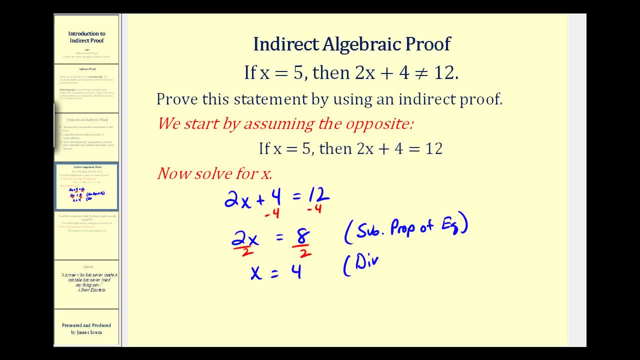 and this was the division property of equality. So, and x equals four contradicts our assumption that if x equals five, two x plus four equals twelve. And this is the key to an indirect proof. Once we reach the contradiction, we can state that our assumption is false. 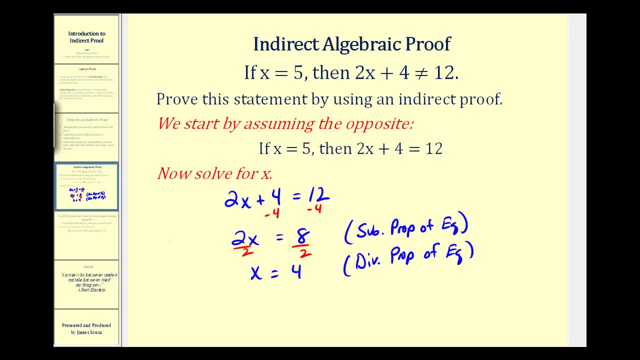 therefore, the original statement must be true. Let's go ahead and write this out: So x equals four contradicts that x equals five. So, as a result, our assumption is false. therefore, two x plus four cannot equal twelve, And this is exactly what we were trying to prove from above. 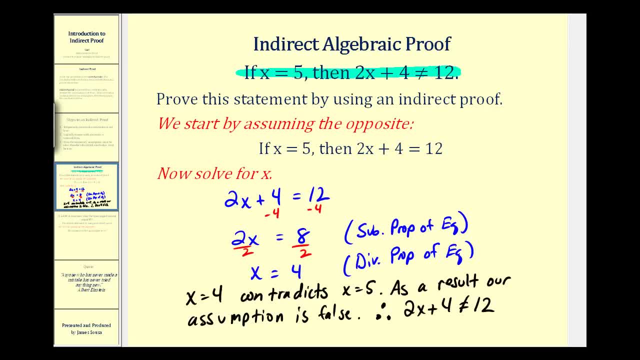 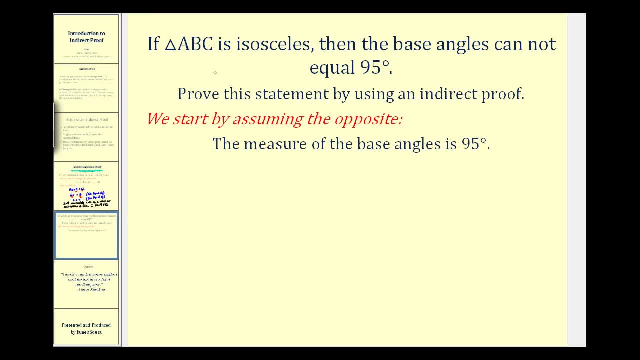 If x equals five, then two x plus four cannot equal twelve. Let's take a look at another example. If triangle ABC is isosceles, then the base angles cannot equal ninety-five degrees. Again, we want to prove this statement by using an indirect proof.